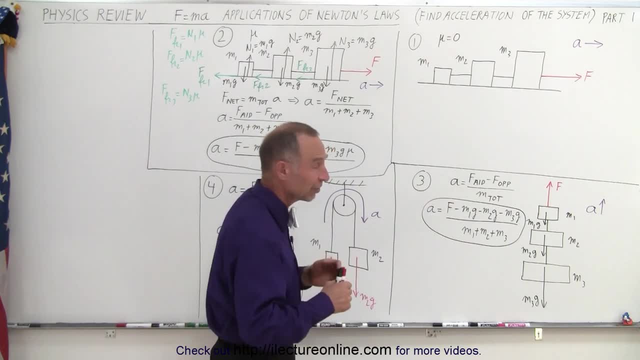 sure. You just pick a side, You say, okay, I think it will accelerate like this, And if you're wrong you'll get a negative answer. So then you can redo it with a different direction. But the first thing you do is assume the direction of the acceleration, draw the diagram of what's. 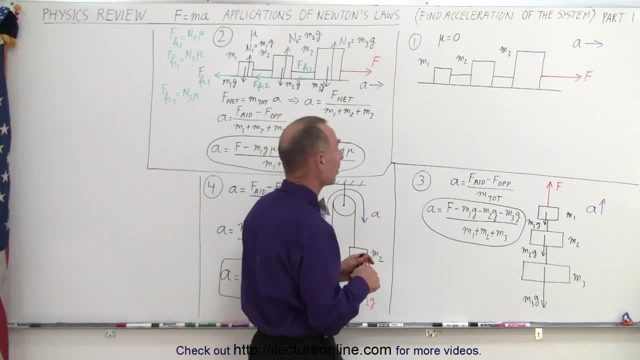 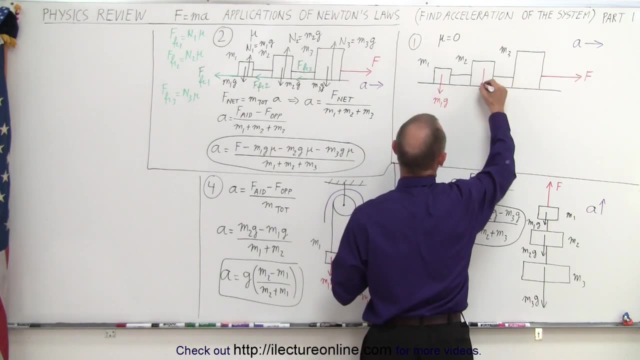 going on And now you need to identify all the other forces that exist there. So we have gravity on it, So we have m1g pointing downward here, We have m2g pointing down here, And we have m3g pointing down here, And then, of course, we have the normal forces, the surface pushing back in. 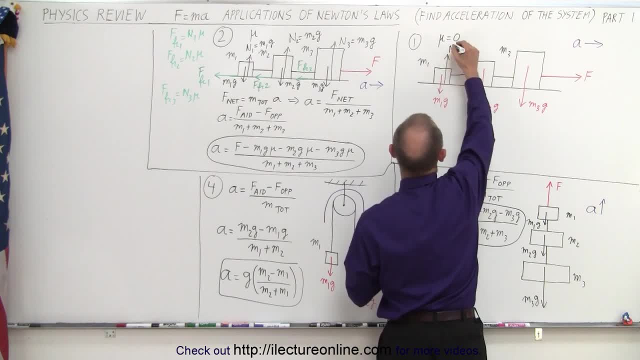 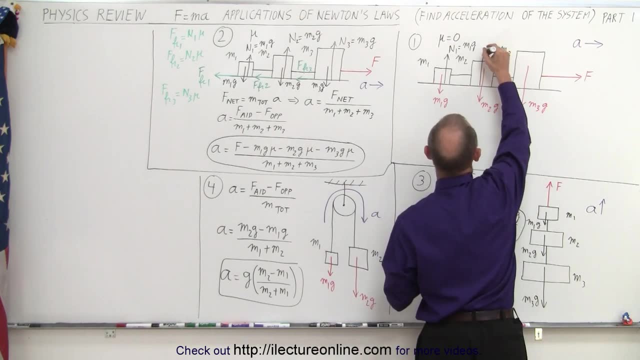 the opposite direction. So here we have n1, and n1 will be equal to m1g. It'll be equal in magnitude but opposite direction to the weight of the object. Here we have n2 pushing back n2, which is equal to m2g. 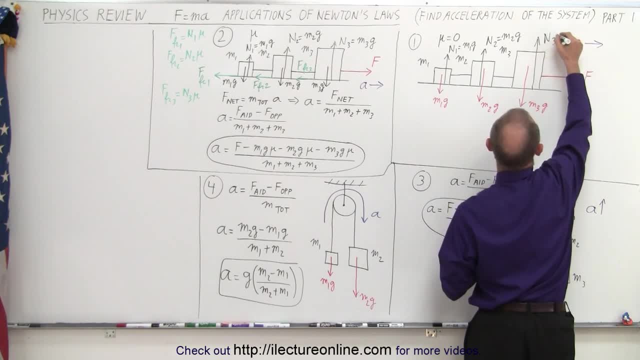 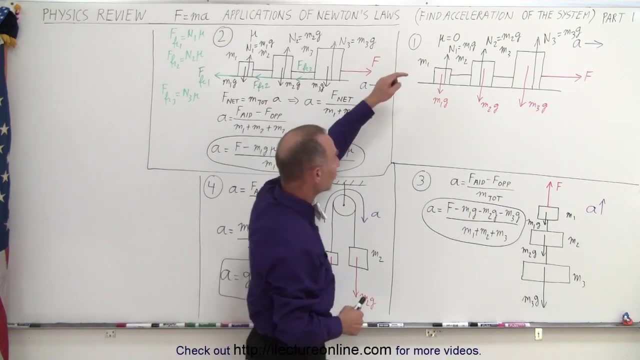 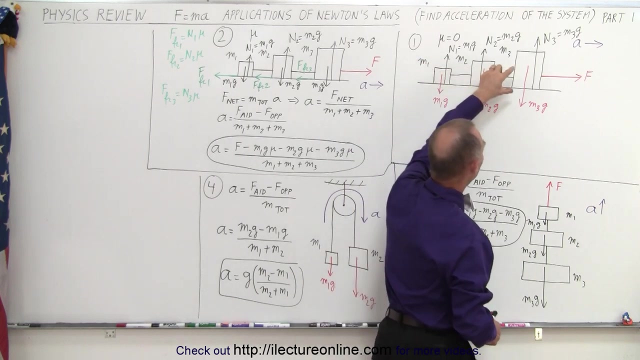 Here we have n3, which is equal to m3g. Now notice that these are three pairs of forces: a force down and a force up. They're equal in magnitude, opposite direction, So essentially they cancel each other out. So does these two and so does these two. So there's no effect on. 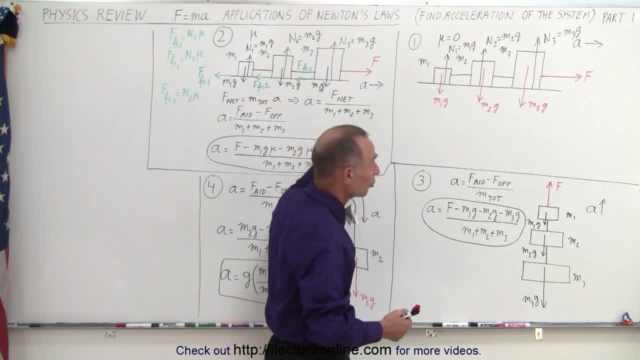 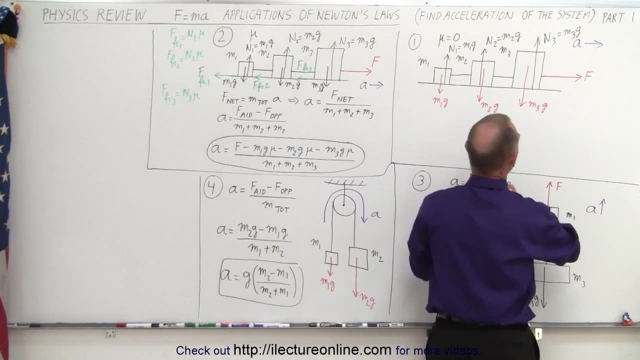 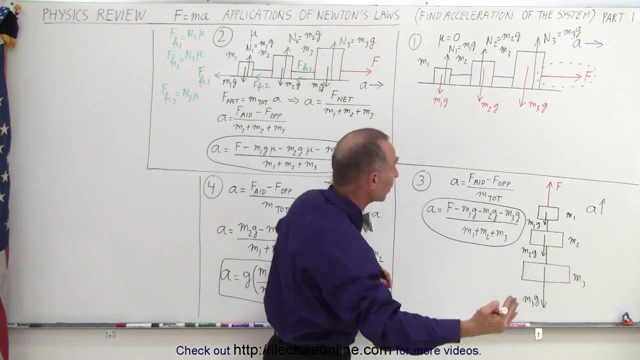 these forces, And besides, they're acting perpendicular to the assumed acceleration, So they can neither add nor detract from the acceleration. The only force left that can actually influence acceleration is this force right here. Now, if there was friction, then of course it would be friction forces pointing in the opposite direction, But in this, 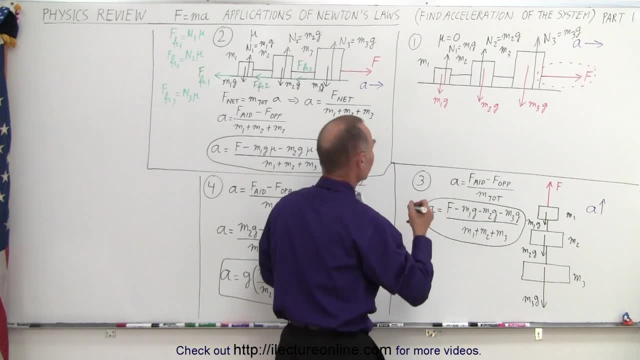 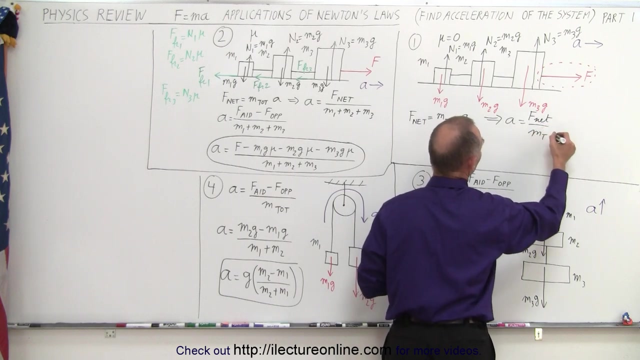 case, there's no friction, But the approach is going to be as follows. We know that f, net- the net force acting on a system, equals the total mass of the system times its acceleration, Which then implies that acceleration is equal to the net force divided by the total mass And the net force. 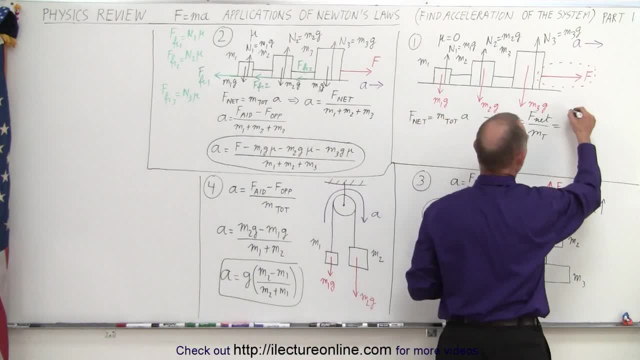 acting on a system times its acceleration minus all the forces opposing the acceleration. So this would be the forces aiding minus the forces opposing, divided by the total mass. In this case there's three masses, So it would be m1 plus m2 plus m3.. So now all we have to do is identify. 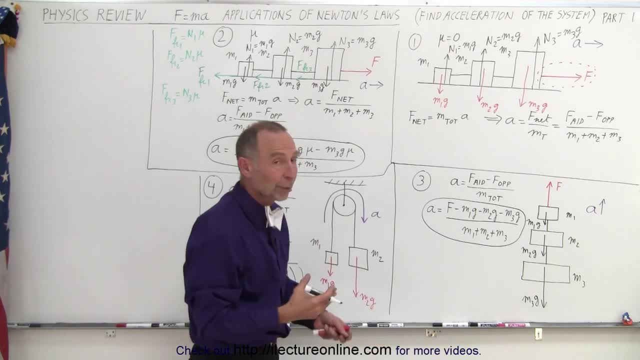 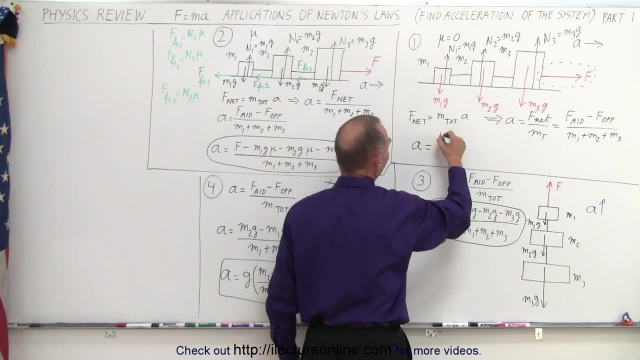 all the aiding forces, then identify all the opposing forces, subtract them from one another, divide by the total mass and we get the acceleration. So here we have acceleration equals. the aiding force would be f and the opposing forces well. there's no forces pointing in the opposite direction, So that would 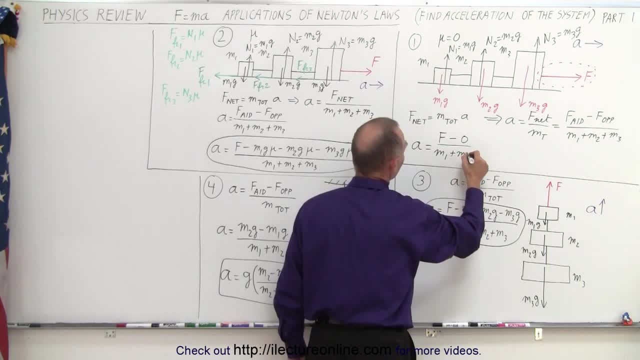 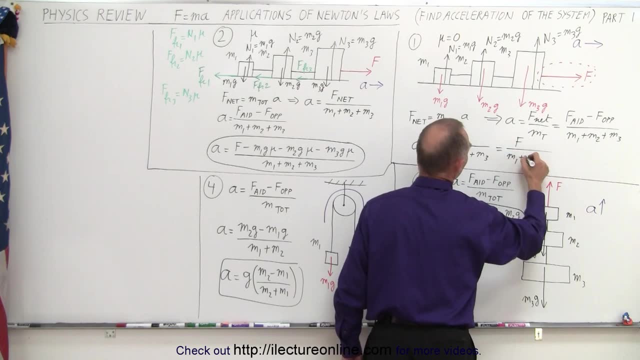 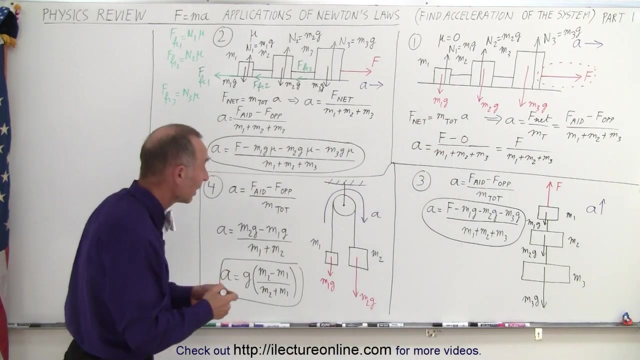 be zero divided by the total mass. So, simplified, that simply means it's the force applied divided by the total mass of the whole system, And that will give you the acceleration of this particular system. Now, what happens if there's friction? Well then, notice that there's going to be a friction. 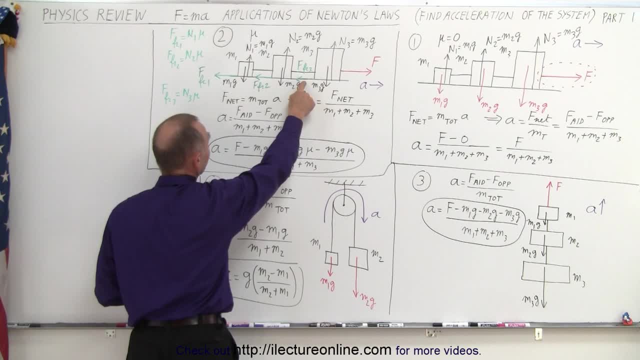 force on the first mass, a friction force on the second mass, a friction force in the third mass and a friction force on the third mass. So by definition the friction forces equal the normal force times mu. So let's say we have mu for all three because we assume that the same material 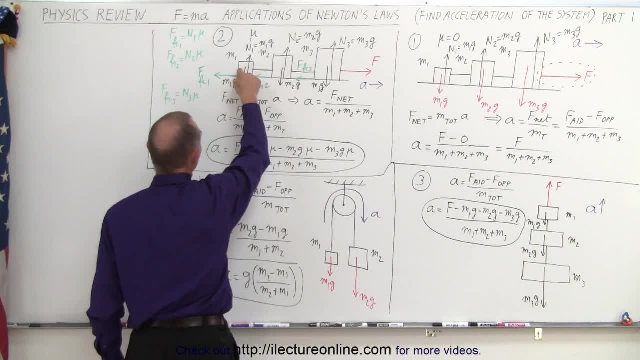 and it's the same floor. So we can see, then, that there's three friction forces: one for the first mass, one for the second mass, one for the third mass, and all three of them point in the opposite direction for the acceleration. So these are opposing forces, while the pulling force is the 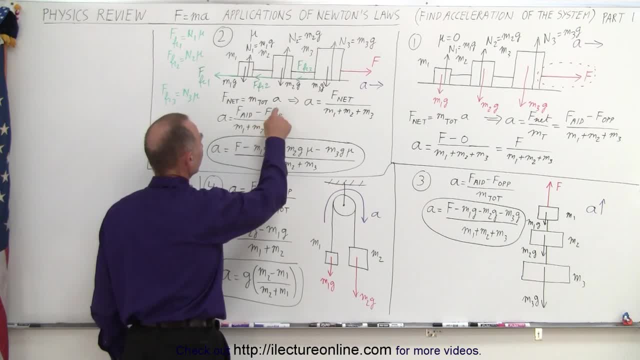 aiding force. That means that the acceleration will be the aiding force minus the opposing force, the three friction forces, The normal force, m1g times mu, m2g times mu, m3g times mu. You subtract them from the aiding force, divide by the total mass, and that will give you the acceleration. 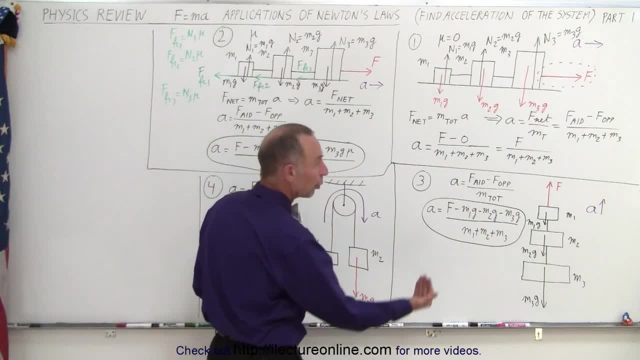 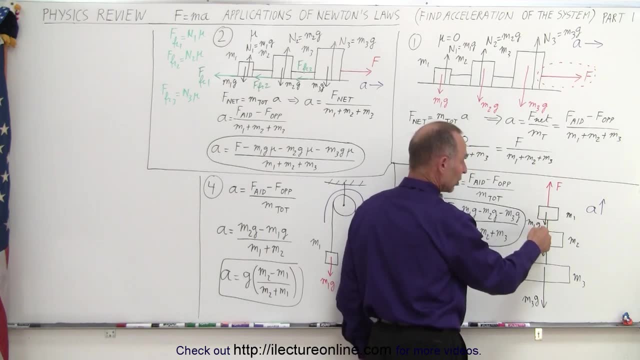 What if we have something that's hanging like this and there's a force pulling all three objects upward? Notice that the objects are connected to one another. Each one of them has a weight: m1g, m2g, m3g. These are the three forces acting downward. 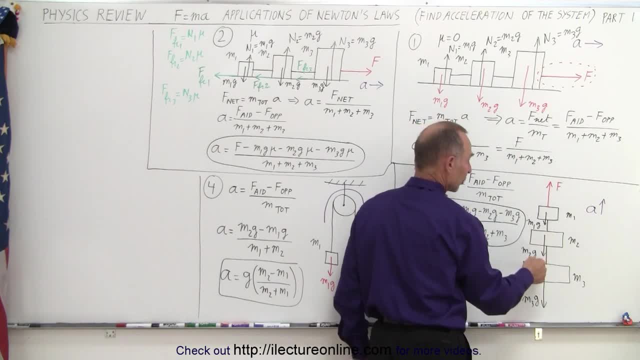 and the one that's hanging is the force that's pulling the three forces downward. And the one that's hanging is the force that's pulling the three forces downward And the one that's acting upward If this force is bigger than the three weights of the three objects. 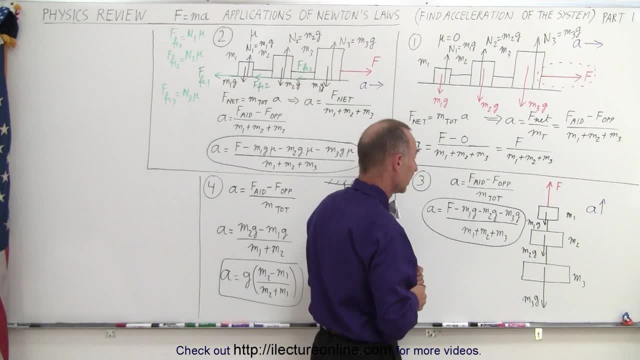 then there will be an acceleration upward. So let's assume it's bigger. So then we can say that the acceleration is equal to the aiding forces minus the opposing forces divided by the total mass. The force that aids is the force in the same direction as acceleration. 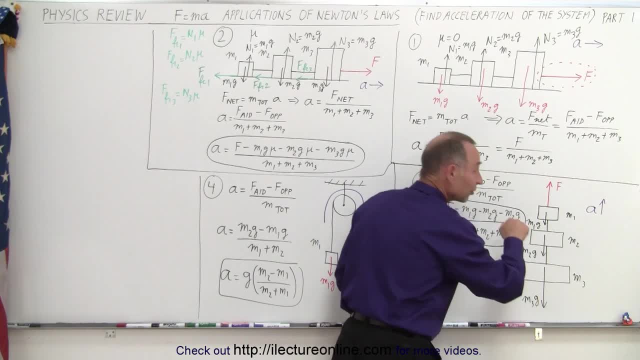 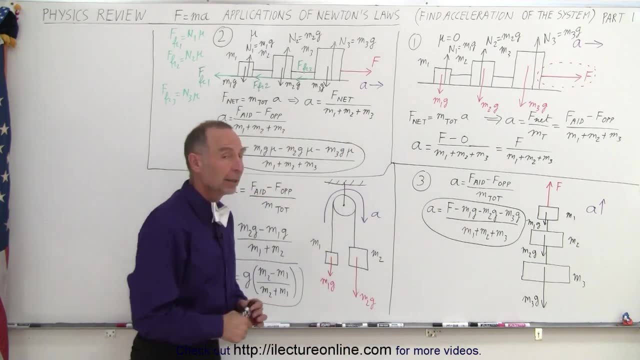 The other three forces need to be subtracted because they're in the opposite direction. they act in the opposite direction relative to the acceleration and you divide by the total mass to get the acceleration. What if we have some thing like this, a pulley, which is also called the Atwood machine? 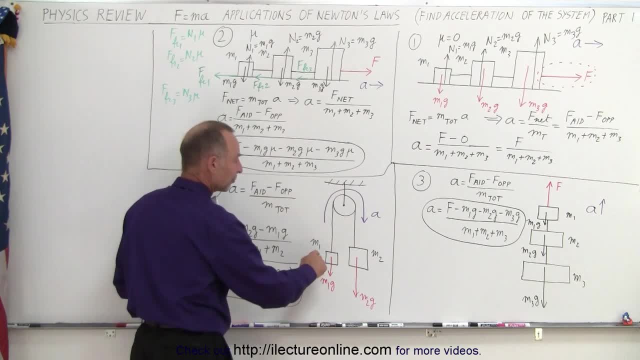 Let's say that the pulley has no mass and no friction. We have two masses hanging on either end. They're attached with a rope going over the pulley And the mass on the right side appears to be bigger than the mass on the left side, which means that its weight is bigger than the one on 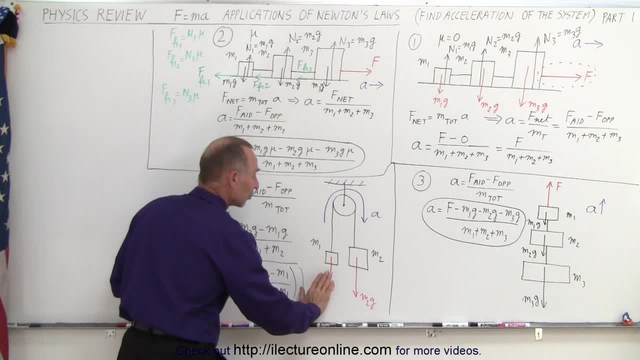 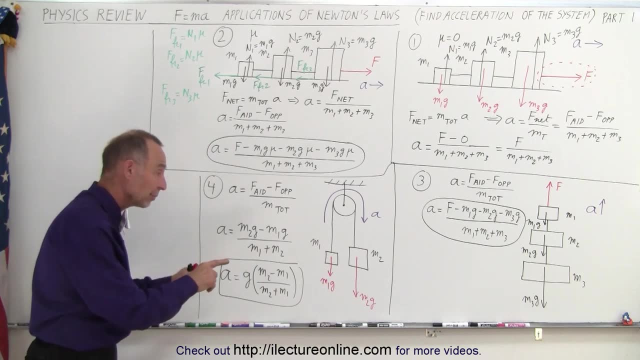 the left side. So we can assume that the acceleration will be such that the small mass will be accelerated upward and the big mass will be accelerated downward. The magnitude of the acceleration for both objects will be the same. The direction is different but the magnitude will be the same. So again, we can use the same principle that 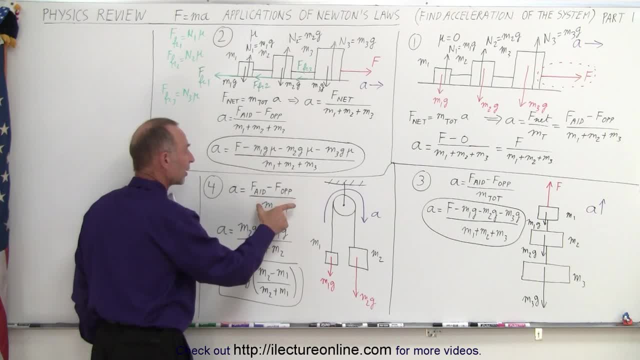 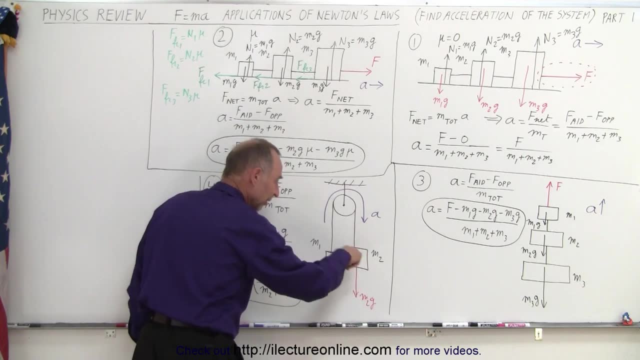 acceleration is equal to the aiding force minus the opposing force divided by the total mass. The aiding force is going to be the force in the same direction as acceleration. M2g acts in the same direction of acceleration. Notice that M1g acts in the opposite direction And you say: 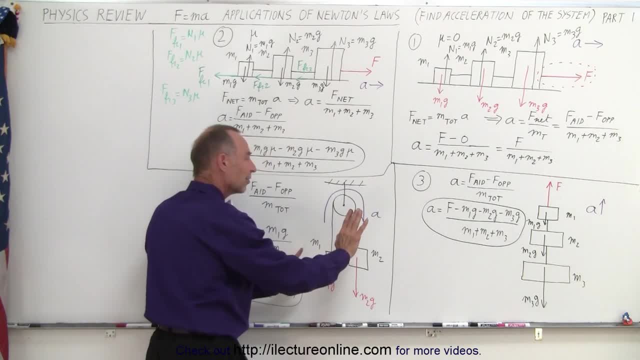 well, wait a minute. M1g also acts downward and aiding, No, no, We have to think about. M1 will be accelerating upward, M2 will be accelerating downward. So if M1 accelerates upward, then M1g pulls in the opposite direction to the acceleration. 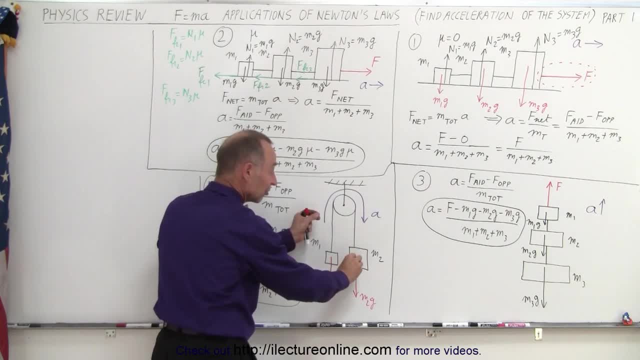 for the system, for this part of the system, But since they're connected, they're essentially a whole system. this force pulls both of these objects to try to make them accelerate this way. This force causes them to accelerate this way. If this is bigger, it will accelerate this way. 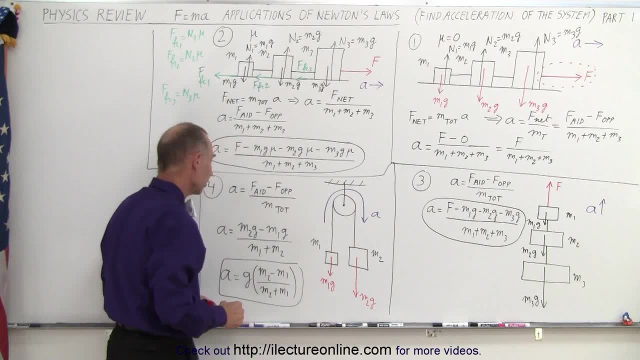 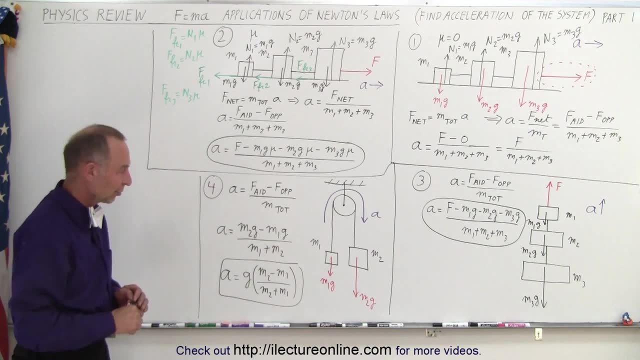 So this is in the opposite direction to the assumed acceleration. So we get M2g minus M1g divided by the total mass. simplified, That will give us the acceleration As shown. And so here's four simple examples. Now we're going to show you some additional. 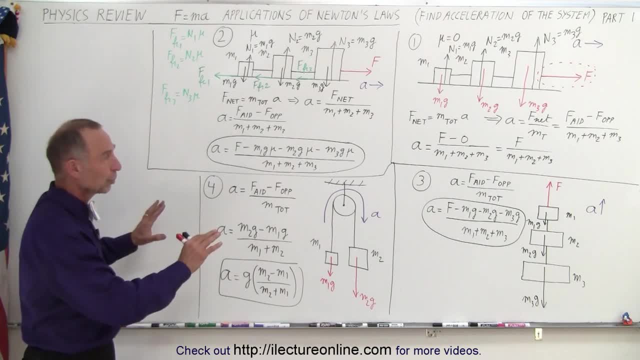 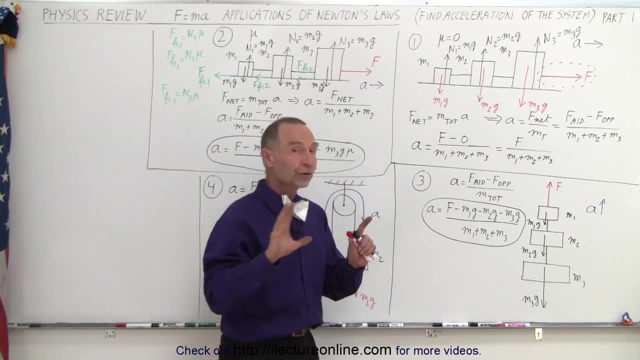 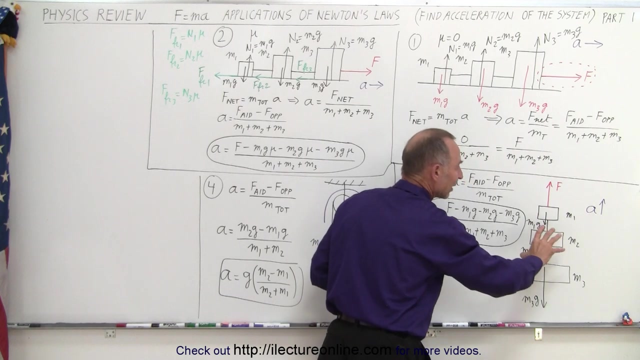 examples that get more and more complicated, But again the approach will be exactly the same. It always will be. F: net equals mass, total times acceleration. All the internal forces are ignored, Notice. we ignore the tension inside the system because those do not add to the acceleration. 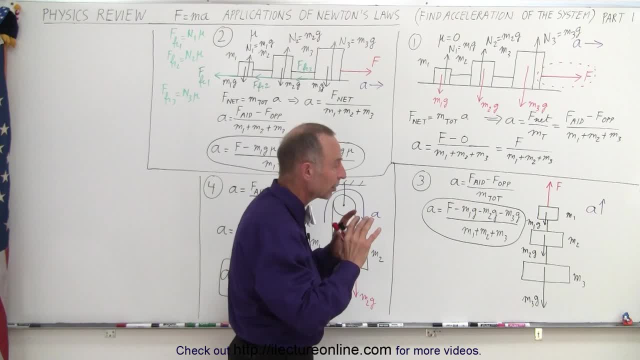 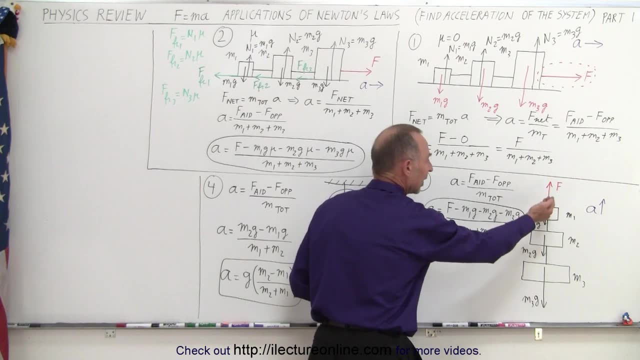 of the system. They just keep the system together. We only consider forces that act on the system and not on the system. So we only consider forces that act on the system From the outside, such as gravity acting from the outside on the three objects and the force acting